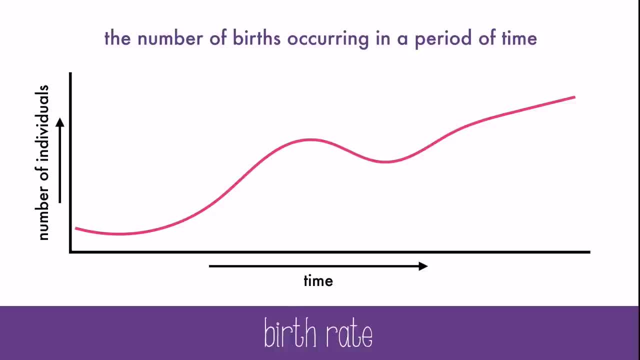 which means the population is likely also increasing. Death rate, or mortality rate, is the number of deaths in a period of time. In this diagram, the death rate is dropping, but what does that actually mean? That means that less people are dying as time goes on. 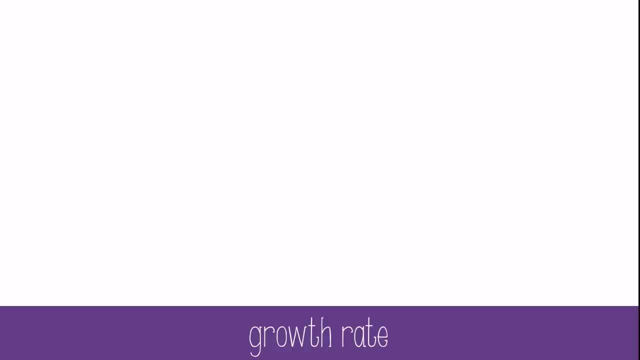 This also means that the population will likely increase. The simple way to find out if a population is growing is to calculate the births minus the deaths. If the number is positive, the population is growing. If the number is negative, the population is shrinking. 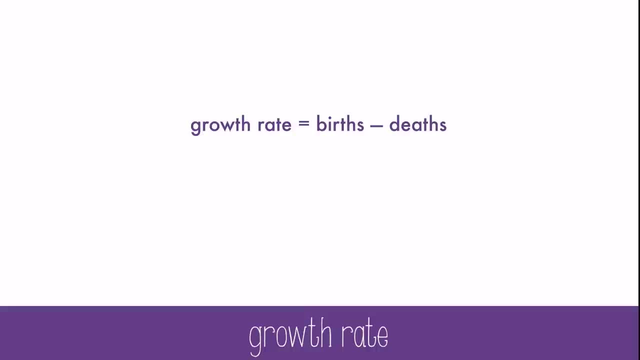 But this is perhaps oversimplified. In reality there's also immigration and emigration to consider. So here's a more realistic growth rate calculation. The growth rate is equal to the births plus the immigration, minus the deaths and the emigration You can remember. 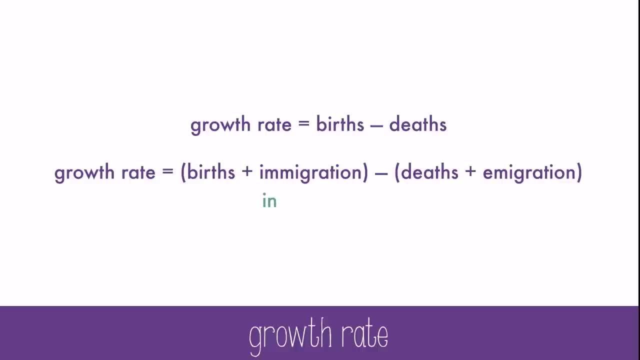 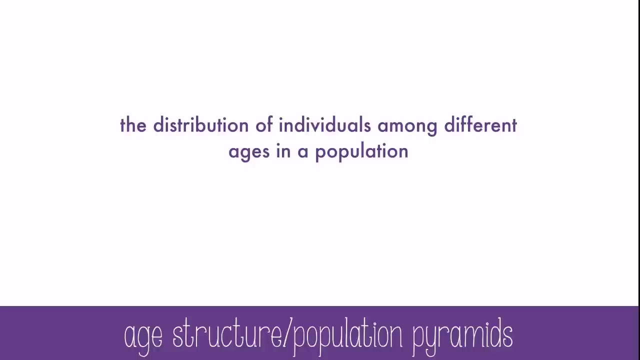 that immigration means individuals coming into a population and emigration is individuals exiting the population. Immigration in, emigration exit. The distribution of individuals among different ages in a population is called age structure. Age structures are often represented in graphs or population pyramids. Let's look at a population pyramid. Here's a population. 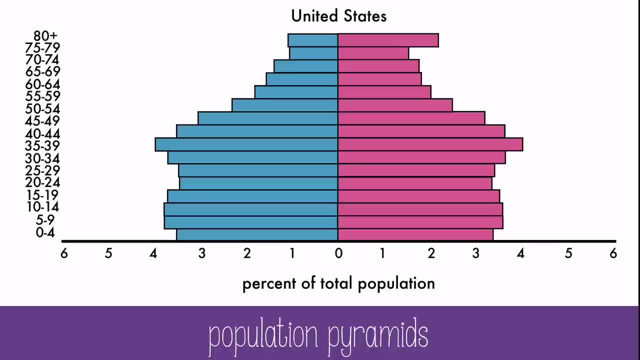 pyramid. for the United States It's fairly stable and it doesn't actually look that much like a pyramid. On the left are the males of the population and on the right are the females of the population. You can see that it's more rectangular than if. 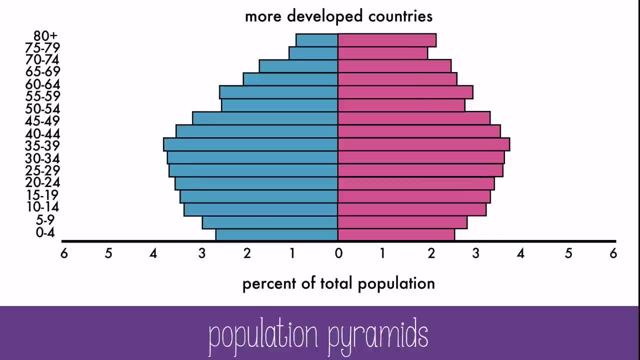 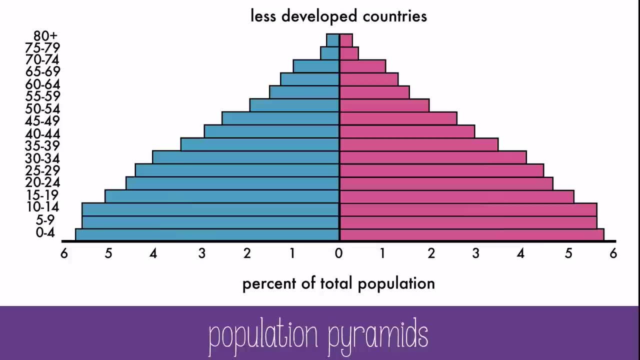 it were, a pyramidal. Here's another developed country. Again, it has more of a square shape than a pyramid. Now, less developed countries tend to have an actual pyramid shape because they have higher growth rates but don't have as many individuals that live to an old age. 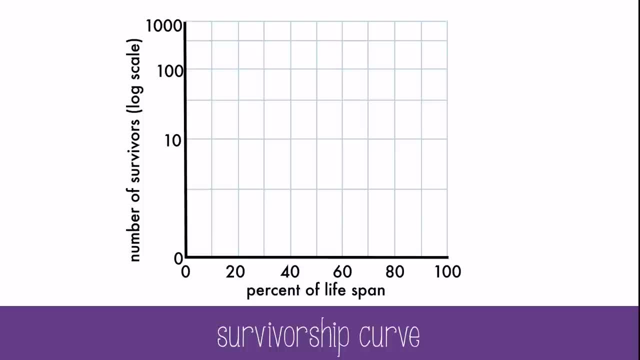 A survivorship curve is a graph that shows the number or proportion of individuals surviving to each age for a given species or group. Type 1 survivorship curves produce few offspring and care for the young. They have high survival rates of the young and they live out most of their expected lifespan and die an old. 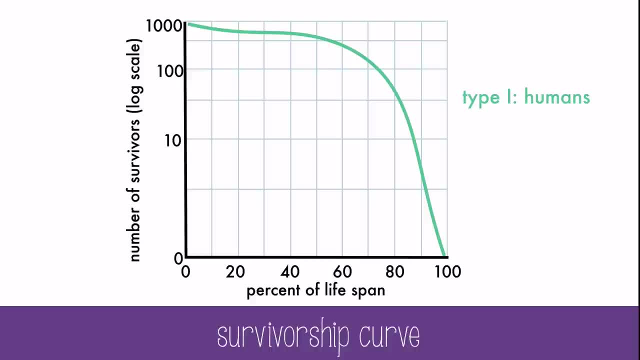 age. Examples of type 1 are humans or even large mammals like elephants. In the type 2 survivorship curve there's a constant death rate throughout the lifespan. An example of this would be coral. Type 3 survivorship curves have many young most. 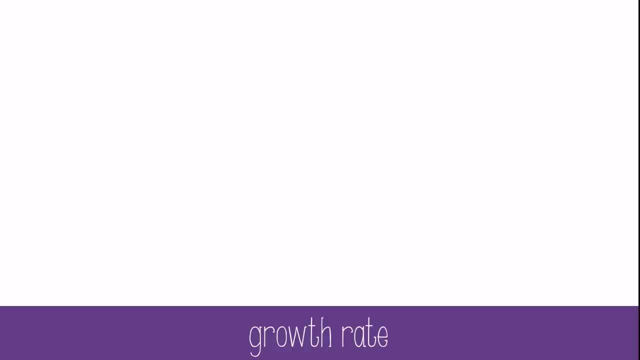 This also means that the population will likely increase. The simple way to find out if a population is growing is to calculate the births minus the deaths. If the number is positive, the population is growing. If the number is negative, the population is shrinking. 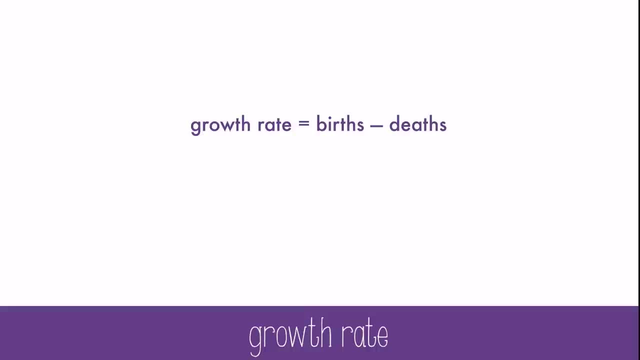 But this is perhaps oversimplified. In reality there's also immigration and emigration to consider. So here's a more realistic growth rate calculation. The growth rate is equal to the births plus the immigration, minus the deaths and the emigration You can remember. 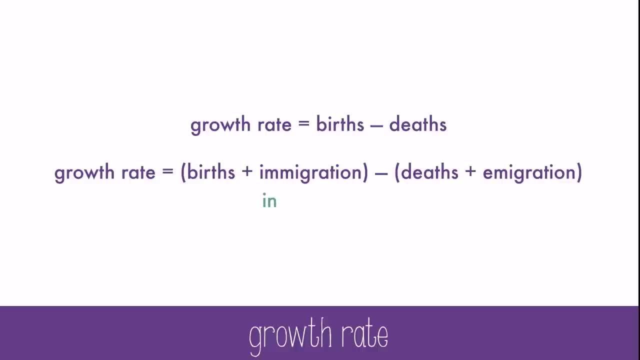 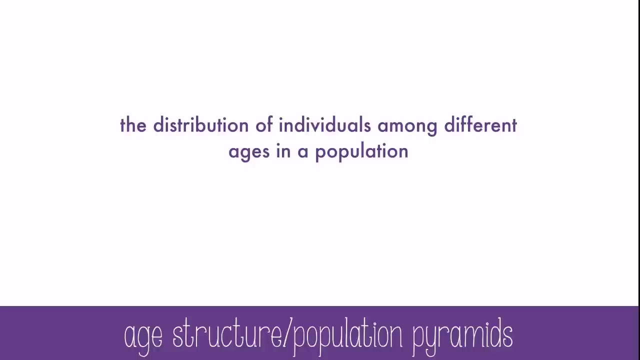 that immigration means individuals coming into a population and emigration is individuals exiting the population. Immigration in, emigration exit. The distribution of individuals among different ages in a population is called age structure. Age structures are often represented in graphs or population pyramids. Let's look at a population pyramid. Here's a population. 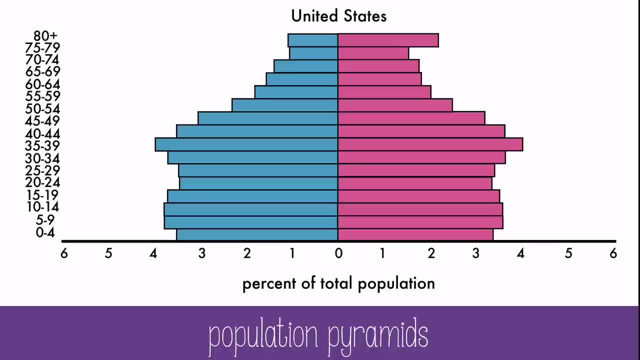 pyramid. for the United States It's fairly stable and it doesn't actually look that much like a pyramid. On the left are the males of the population and on the right are the females of the population. You can see that it's more rectangular than if. 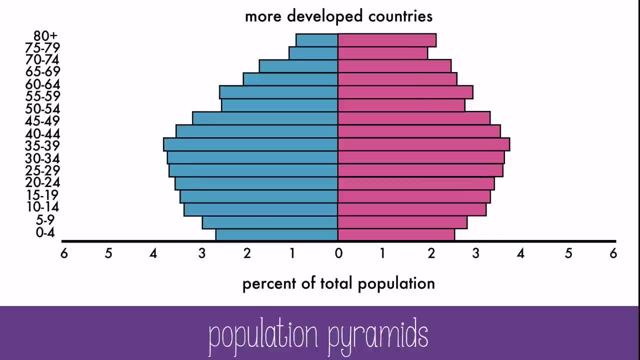 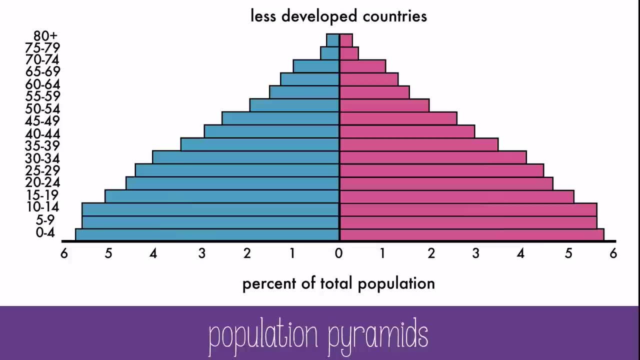 it were, a pyramidal. Here's another developed country. Again, it has more of a square shape than a pyramid. Now, less developed countries tend to have an actual pyramid shape because they have higher growth rates but don't have as many individuals that live to an old age. 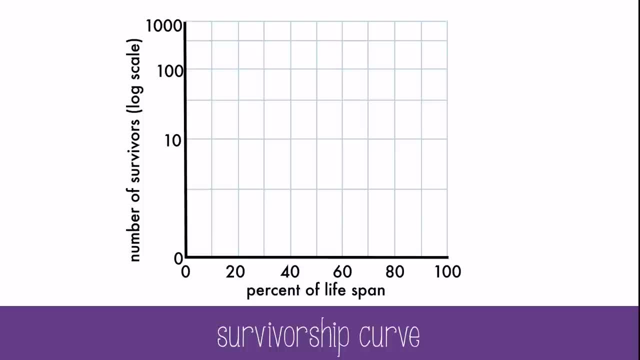 A survivorship curve is a graph that shows the number or proportion of individuals surviving to each age for a given species or group. Type 1 survivorship curves produce few offspring and care for the young. They have high survival rates of the young and they live out most of their expected lifespan and die an old. 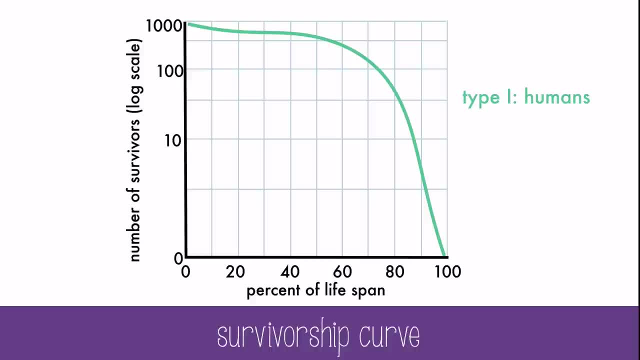 age. Examples of type 1 are humans or even large mammals like elephants. In the type 2 survivorship curve there's a constant death rate throughout the lifespan. An example of this would be coral. Type 3 survivorship curves have many young most. 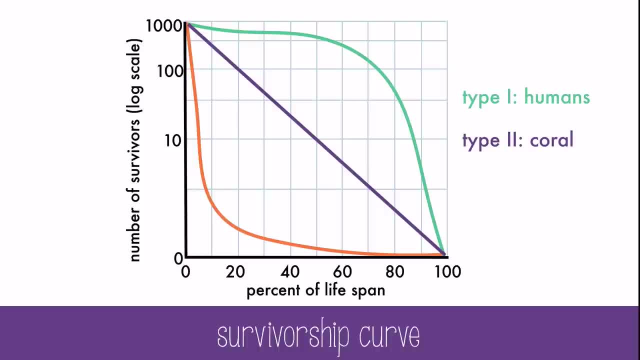 of which will die at a very young age. An example would be plants. They make lots of seeds, but very few of them will actually make it into adults. Now, each of these types of survival have their benefits and their drawbacks. For example,